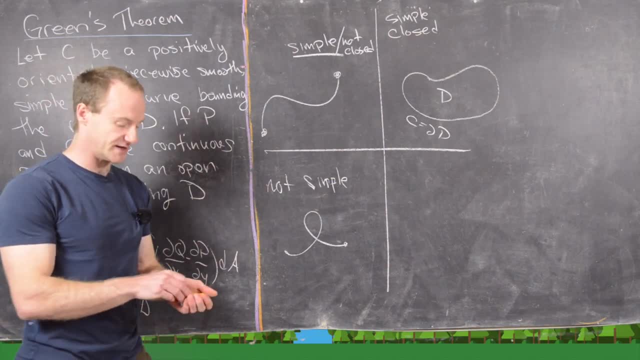 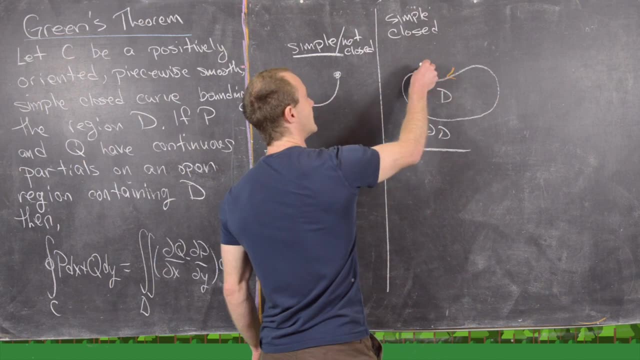 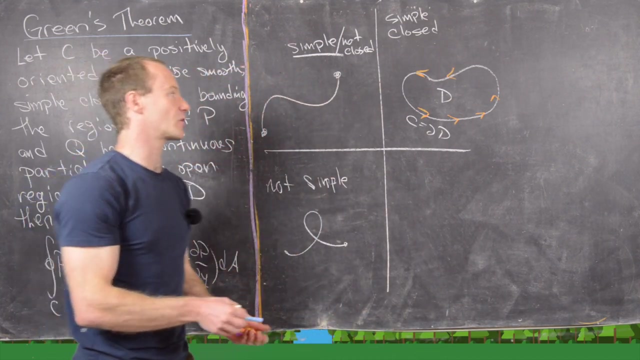 that covers everything except for positively oriented. So positively oriented means you have parameterized the curve in a way so that if you walk in the direction of the parameterization, the region is on your left. So notice, if we were to walk along that curve, the region D would be. 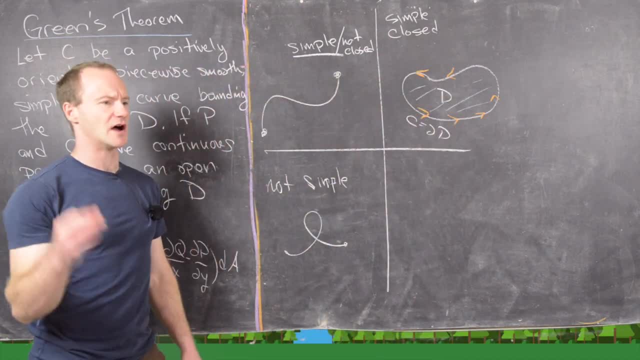 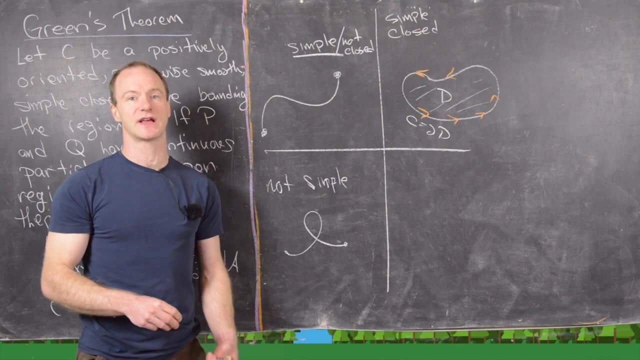 on our left, And so this is, in general, like a counterclockwise parameterization. Okay, so now let's go ahead and clean up the board, and then we'll do a very special case of the proof. Okay, so now we're going to look at a very special case of the proof of this theorem, and that case is: 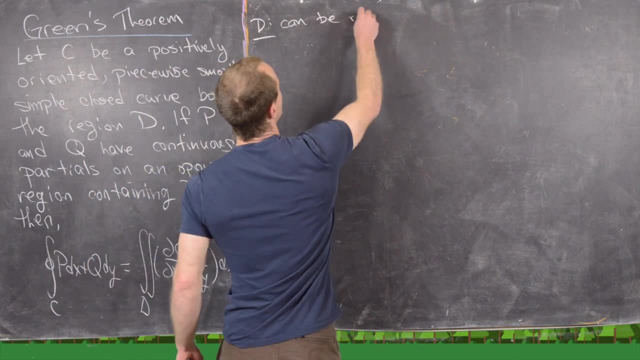 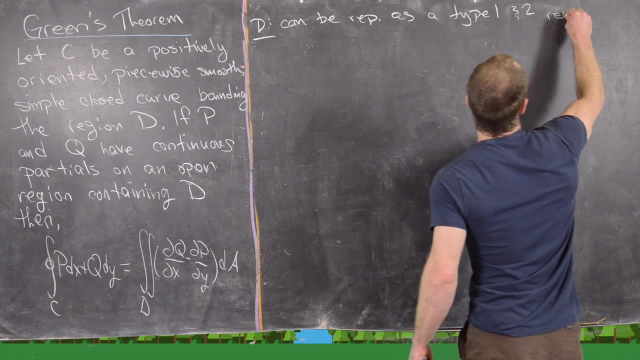 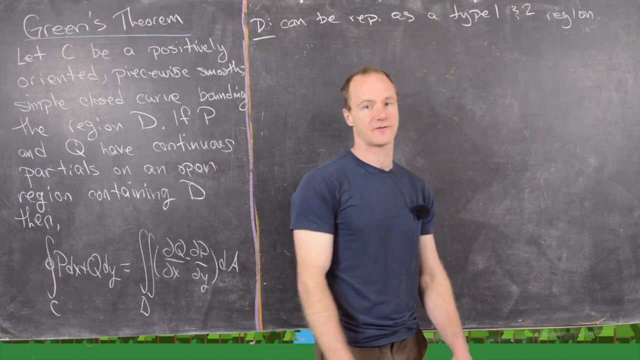 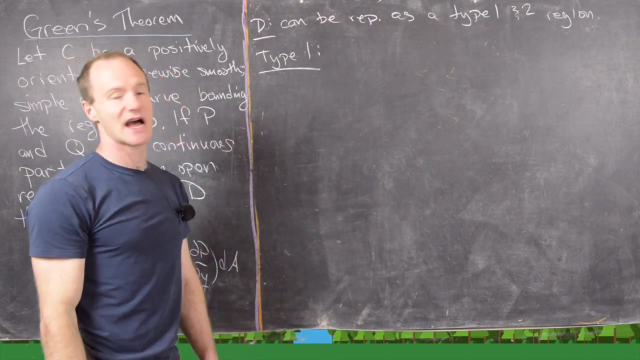 the following: So D can be represented as a type 1 and 2 region And you see, we'll get half of this equality from the type 1 region and the other half from the type 2 region. So let's first look at representing D as a type 1 region, which means D can be written as the coordinates. 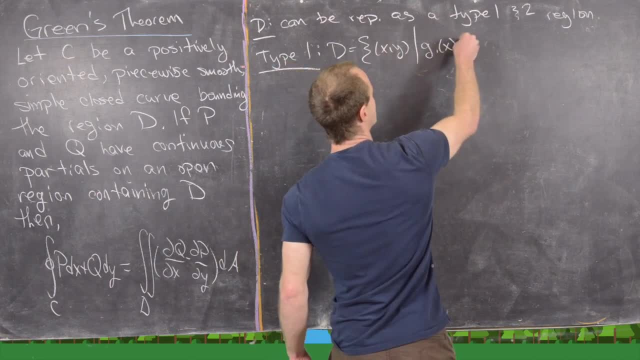 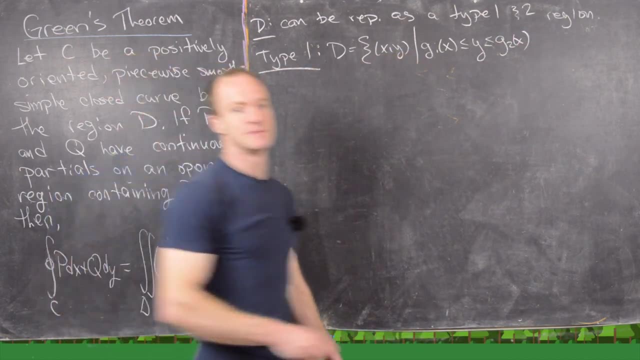 x and y, And here x is going to be between two functions of x, and I should have said y is between two functions of x, And then x is going to be between two functions of x, and then x is going to be is between two numbers, A and B. 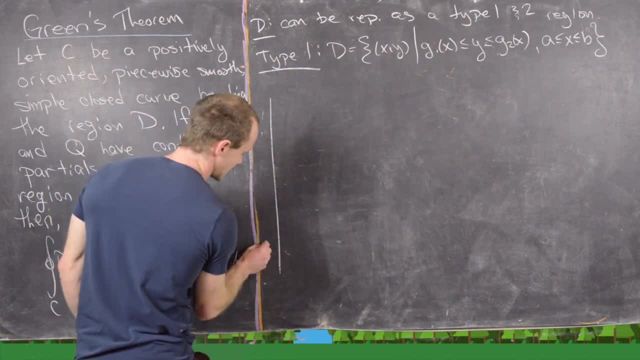 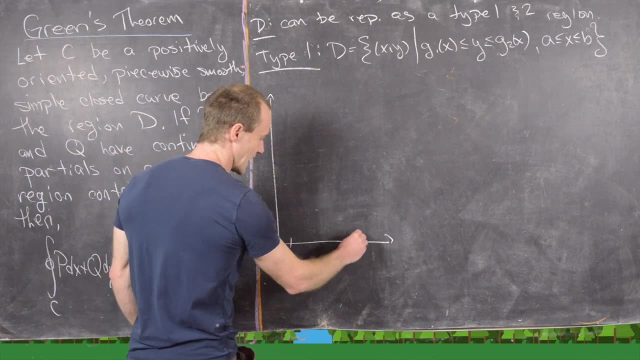 Okay, so let's go ahead and draw a picture of what that looks like. I'll put it all in the first quadrant, although obviously this could be much more general. So let's say: here is our point A, here's our point B. 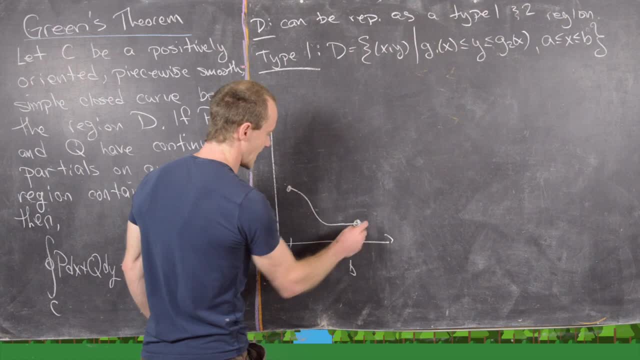 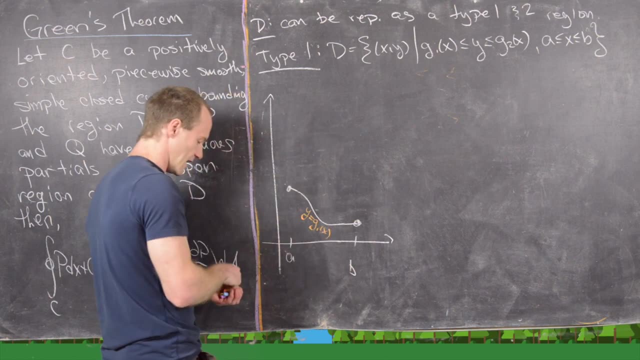 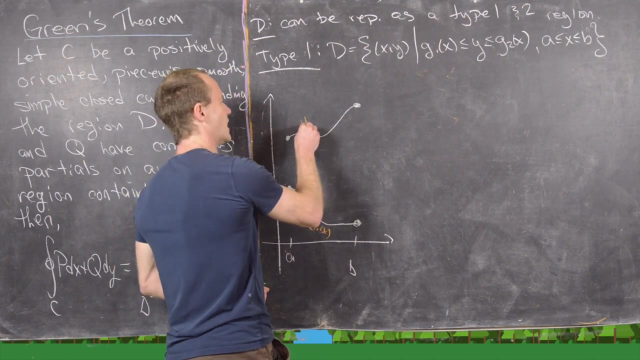 We could make our curve G1, do something like that, So I'll go ahead and call this thing: Y equals G1. And then we could make G2.. Do something like that, So I'll go ahead and call this thing: Y equals G2 of X. 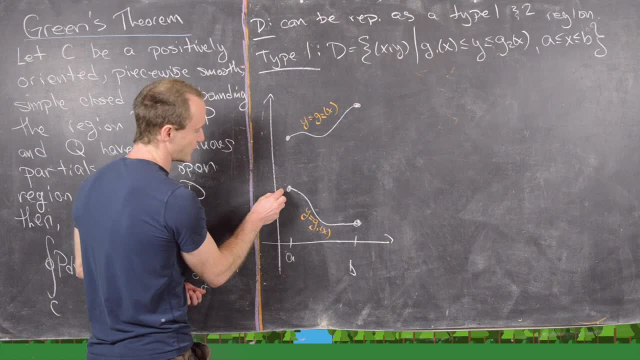 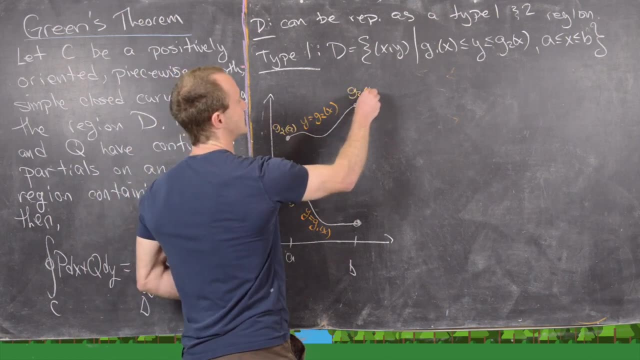 And then notice, these points at the corner are gonna be pretty important, So I'll call this G1 of A. up here will be G2 of A, This is G2 of B and then down here is G1 of B. Great, 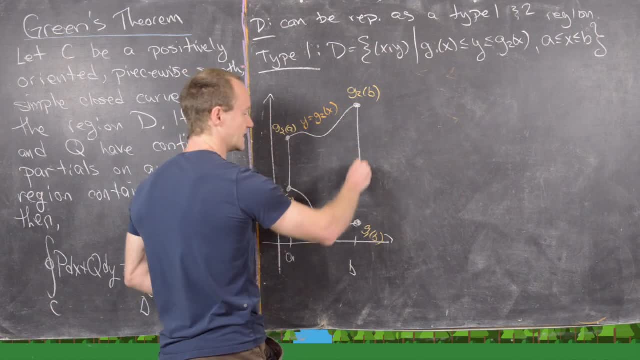 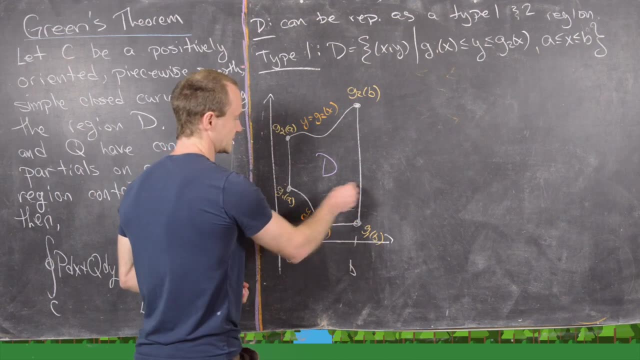 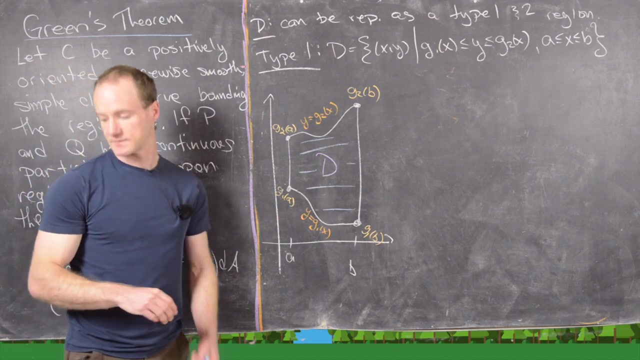 And then, also important, are these vertical lines connecting these points. So that makes our region D inside here, like this, Great. And now let's give some names to these boundary curves. So we could call this one C1,. we could call this one C2,. 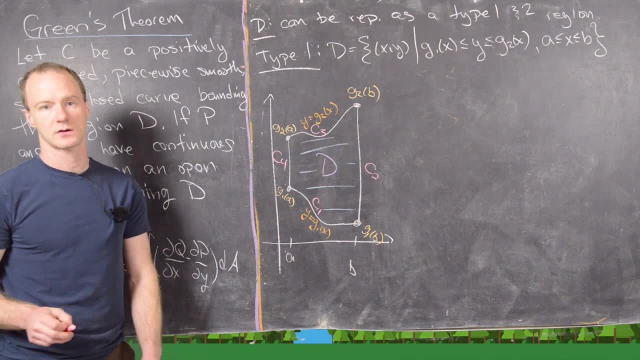 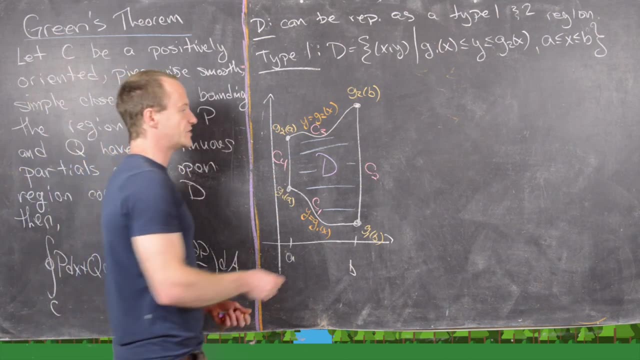 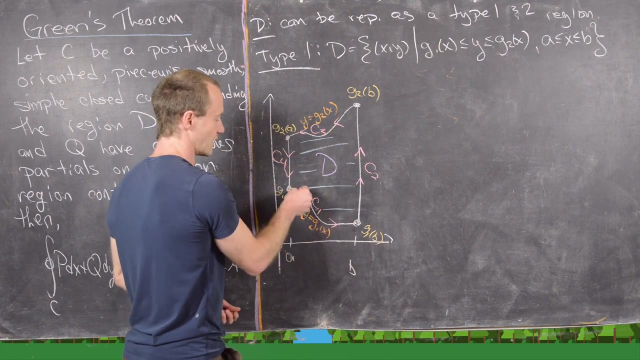 we could call this one C3, and we could call this one C4. And then if we wanna orient this so that it's positively oriented, then we should orient it. so we're going up along this curve, left along this curve, down along this curve and right along this curve. 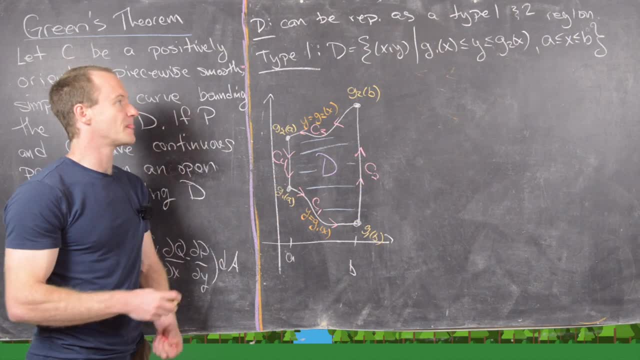 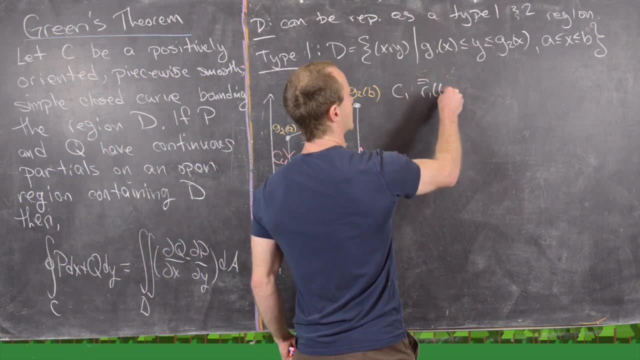 And notice that will put the region D to our left. And now let's parametrize each of these curves. So notice C1 can be parametrized in the following way: So R1 of T, we'll write this as a vector equation. 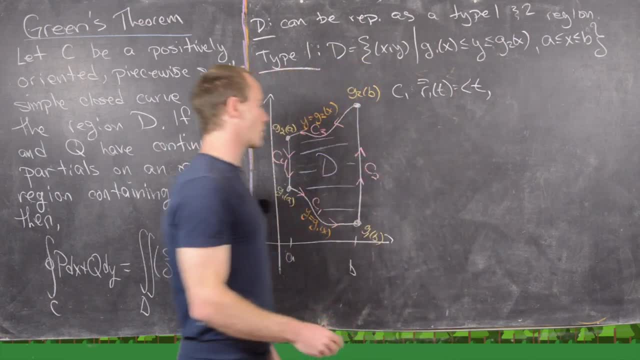 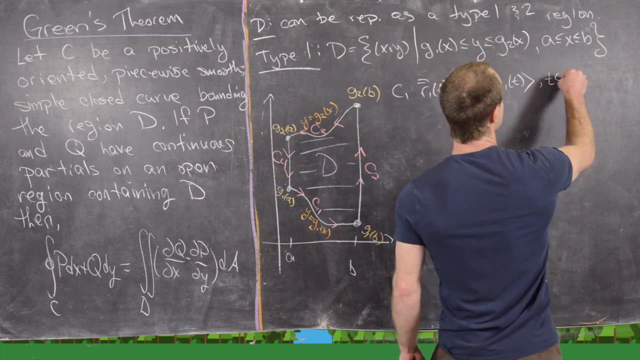 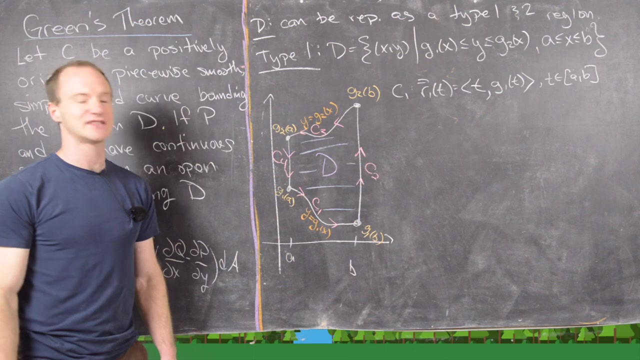 So notice, we can take T to be the X coordinate, and then we can take G1 of T to be the Y coordinate, And then T. T is going to range between A and B. Good, so that will start here and it'll end there, just as needed. 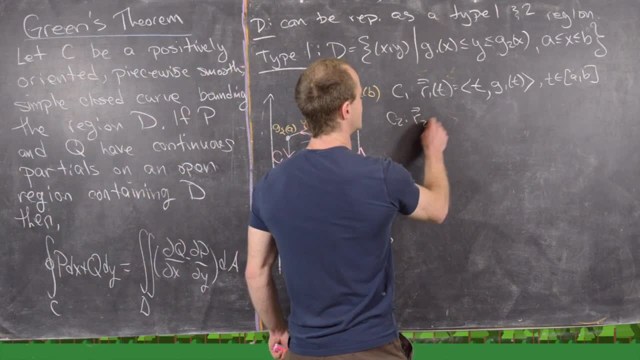 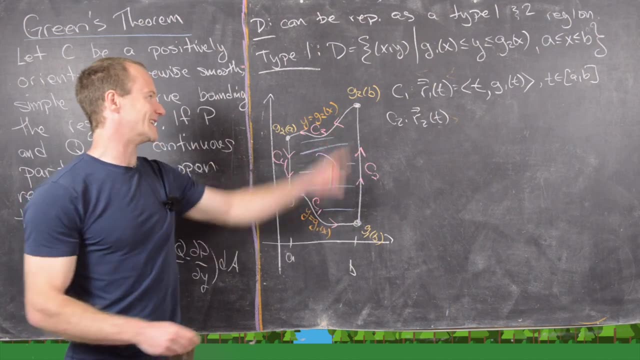 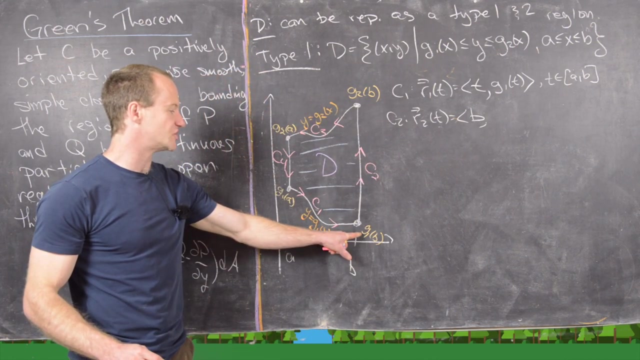 Now let's look at C2.. So notice C2, we can parametrize with this thing: R2.. And here the B- sorry, the X coordinate is fixed at the number B, And then the Y coordinate is trending between G1 of B and G2 of B. 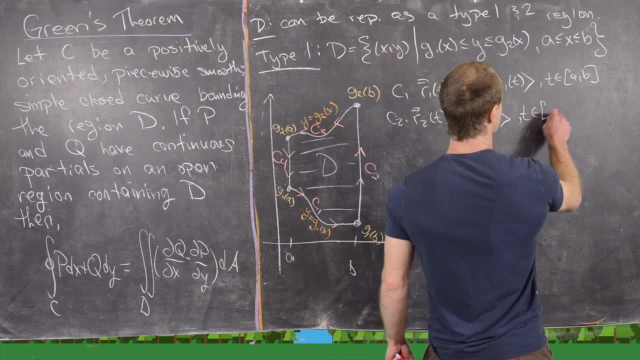 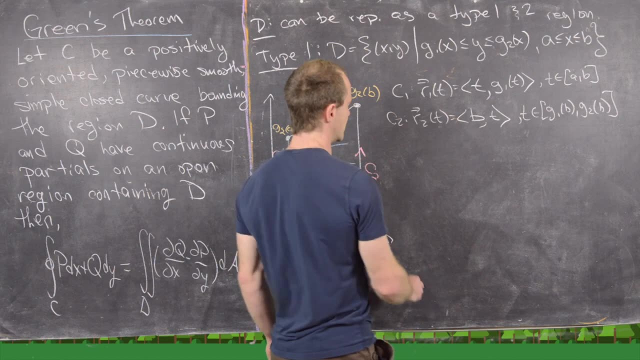 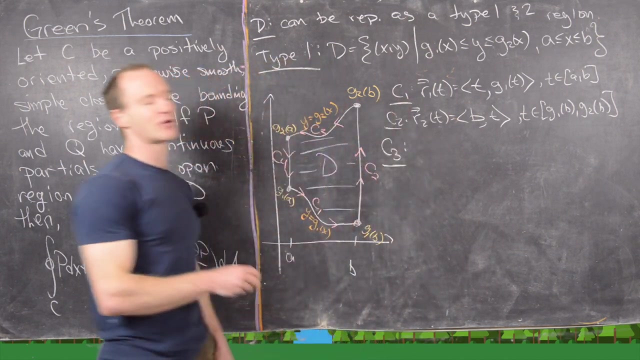 So maybe we could say that's T, and then now T is going between G1 of B and G2 of B, like that Good. And now let's look at C3.. So C3, so that'll be this top curve right here. 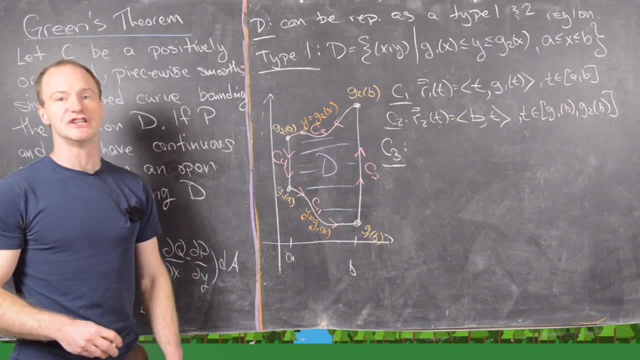 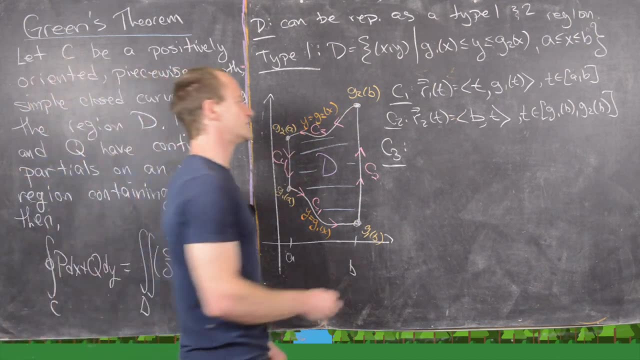 So notice again, we're on the plane. curve Y equals G2 of X, kind of similar to what we did here before, but we're going in reverse. So I'm actually gonna abuse notation in this case And I'll essentially write the same thing. 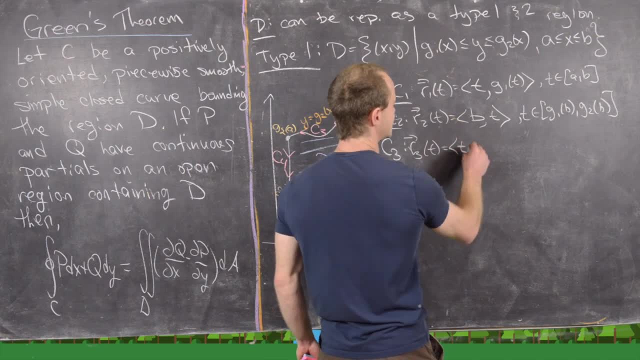 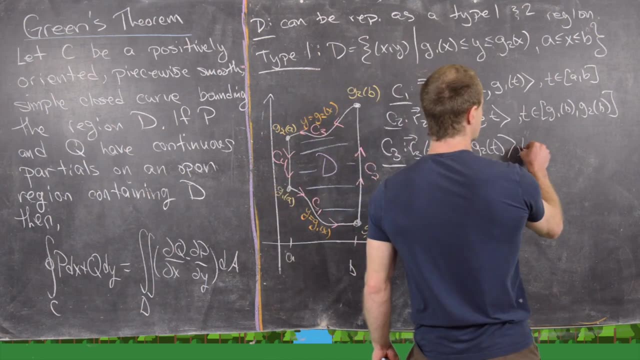 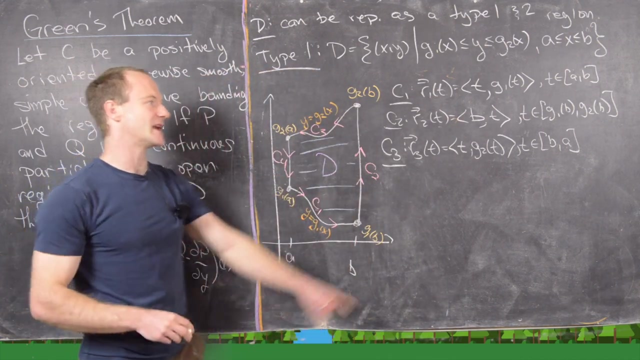 that we had for R1.. I'll say: this is T G2 of T. Notice that's gonna put us on this curve, but we wanna go in reverse, which means we want T to start at B and go to A. Okay, so now that doesn't really make any sense. 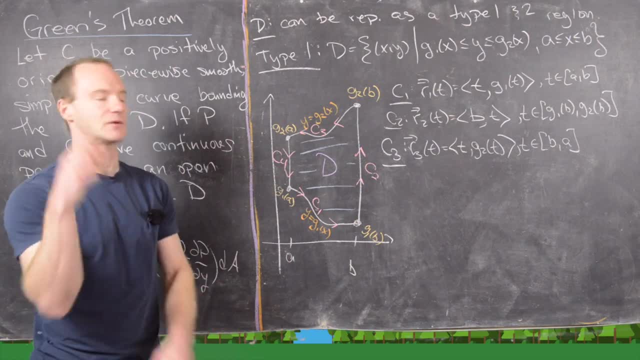 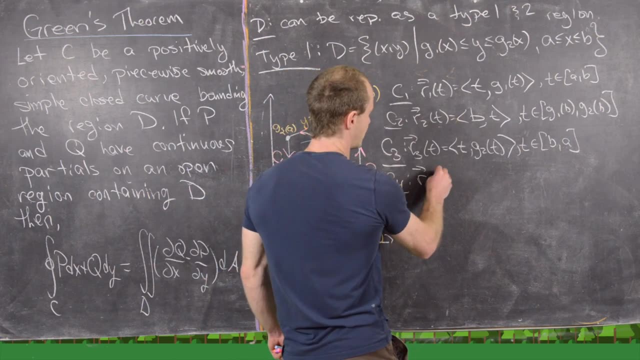 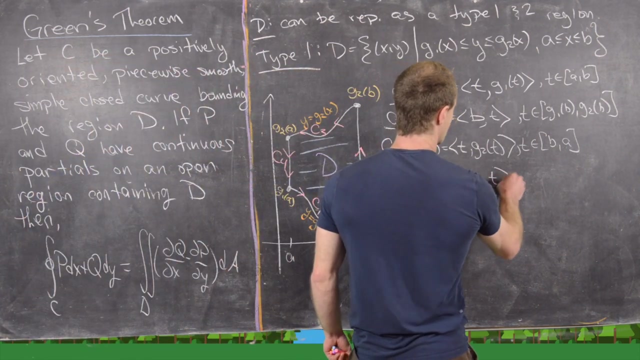 as an interval, but if we interpret it as just reversing this thing, then we're okay. Okay, so next we want C4, which is gonna be R4 of T. Notice, the X value is fixed at A And then the Y value will run between G2 of A. 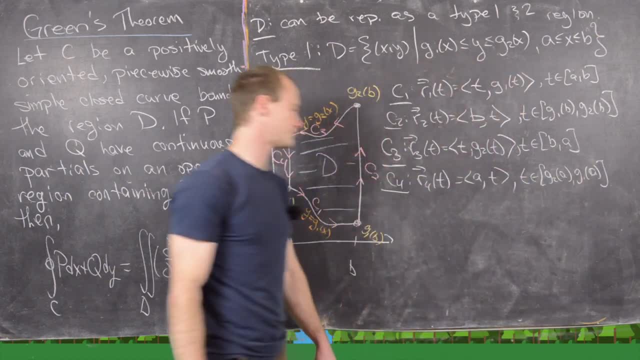 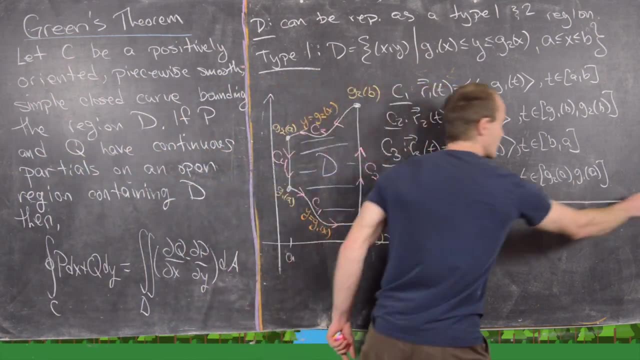 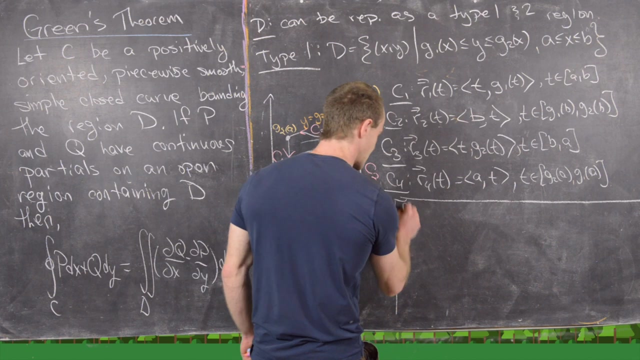 and G1 of A, just as before. Okay, great. So now we're actually all set in order to show that our Green's theorem is starting to be built out of this process. So let's go ahead and take the double integral over D. 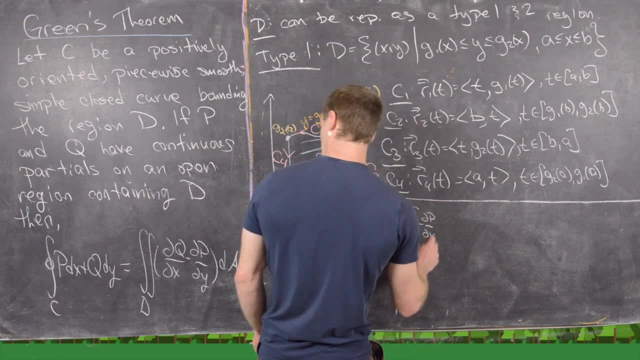 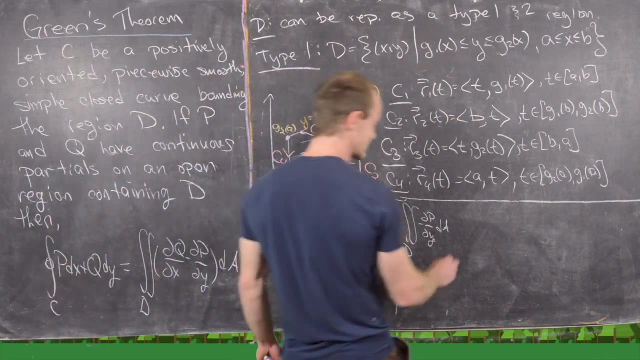 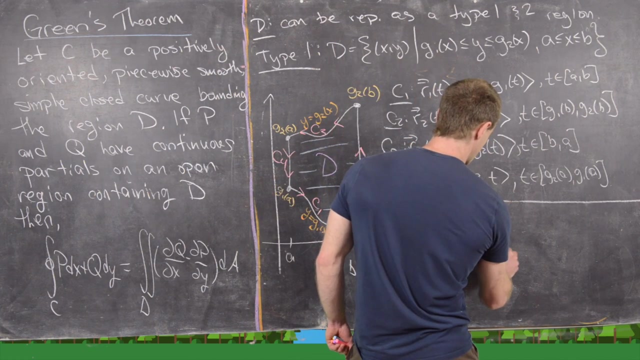 of minus DP DY DA. Okay, so since this is a type one region, we can write this as the integral from A to B, the integral from minus- sorry- from G1 of X to G2 of X, and then we have minus DP DY DY. 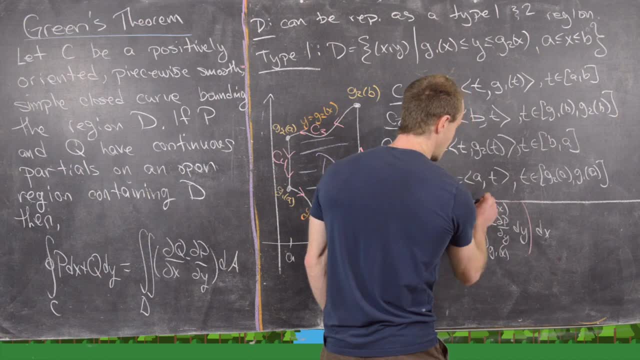 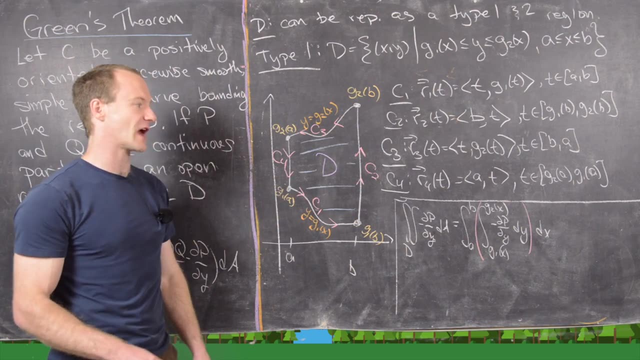 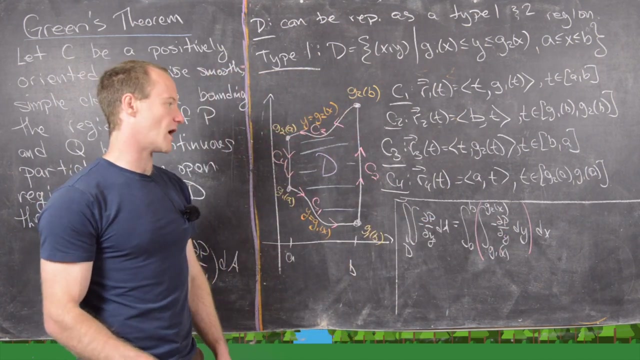 Y, DX, and I'm gonna go ahead and put in pink parentheses that inner most iterated integral. But now we can apply the fundamental theorem of calculus to that inner integral and have the partial with respect to Y cancel with this Y. And also, maybe, before we do that, 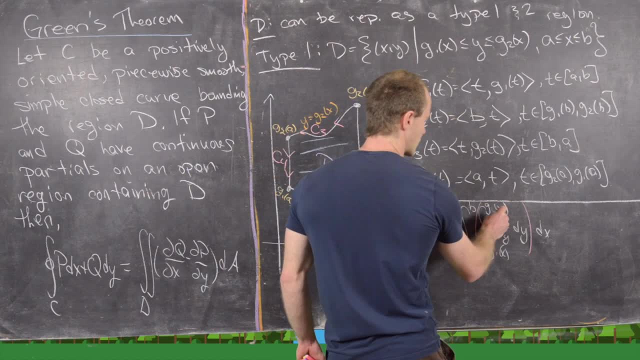 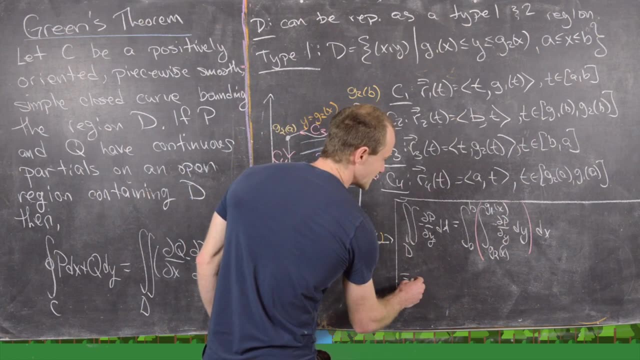 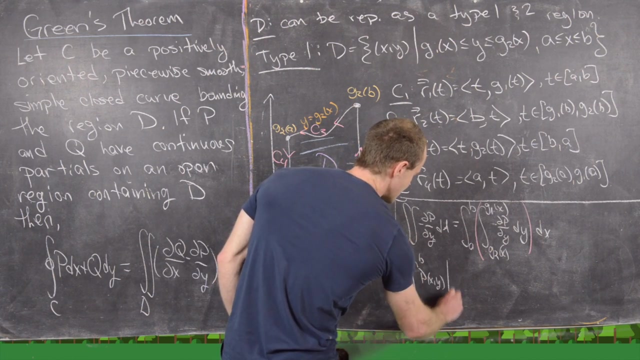 let's take this minus sign and use it to change the order of the bounds of integration. So now G2 is on the top and G1 is on the bottom. Okay, so that's gonna give us the integral from A to B of the function. P of XY, evaluated from Y, equals G2 of X. 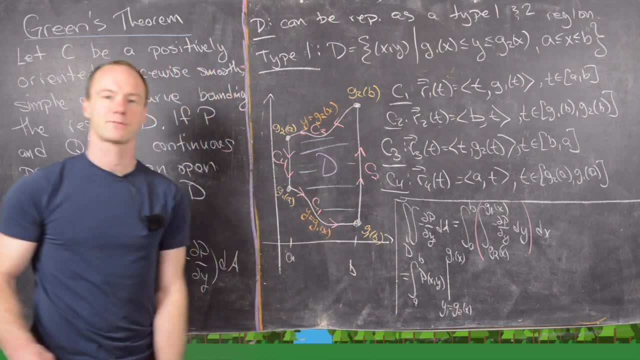 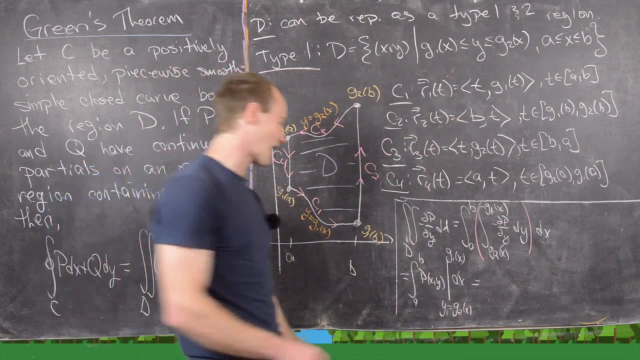 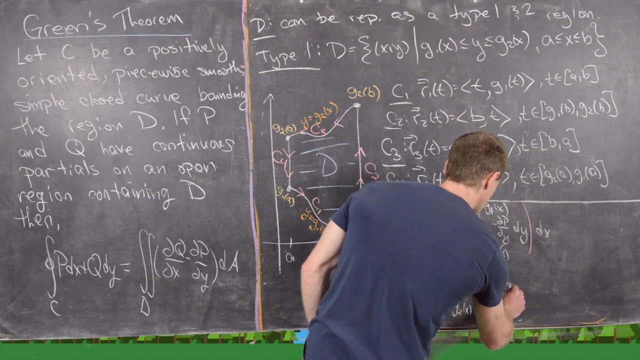 all the way up to Y equals G1 of X, like that. Okay, but now we can write that DX. but notice this is exactly equal to the integral from A to B of P of X. So that's gonna be X, G1 of X minus P of X, G2 of X, DX. 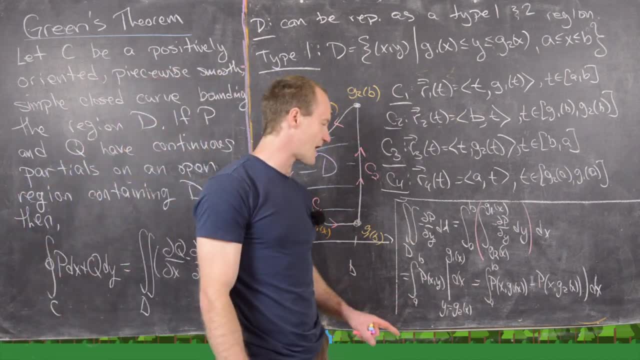 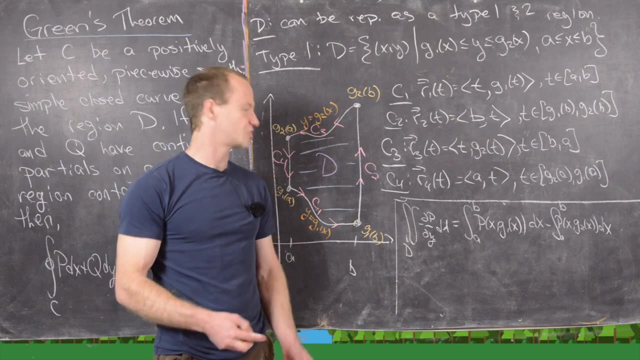 Okay, good, So now we're running out of room, but we actually don't have much, So I'm gonna erase these couple of steps in the middle and bring that up, and then we'll finish this off. Okay, so just previously we had gotten it down to this point. 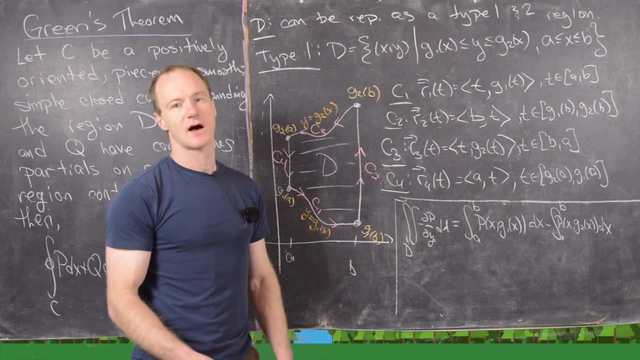 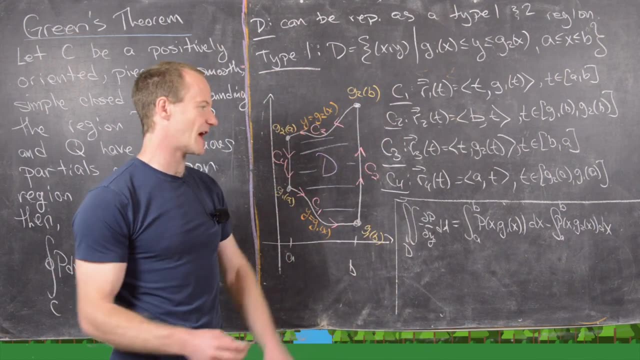 so we have the integral from A to B of P of X, p of x, comma g1 of x dx, minus the integral from a to b of p of x, comma g2 of x dx. so i split that into two integrals. now the next thing that i want to do is maybe let's go ahead and replace the x's. 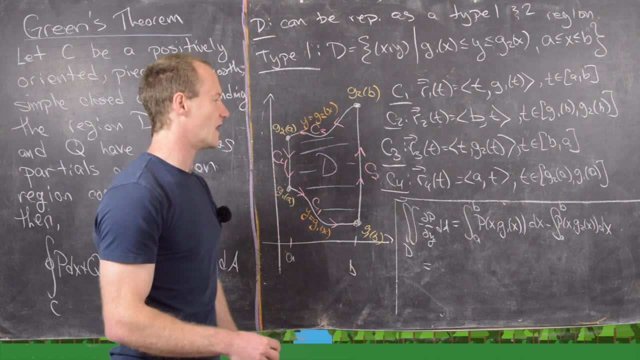 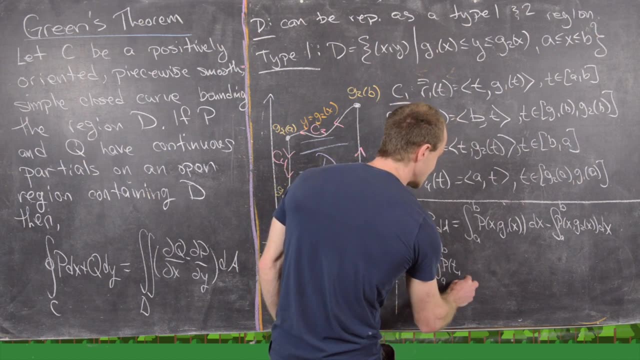 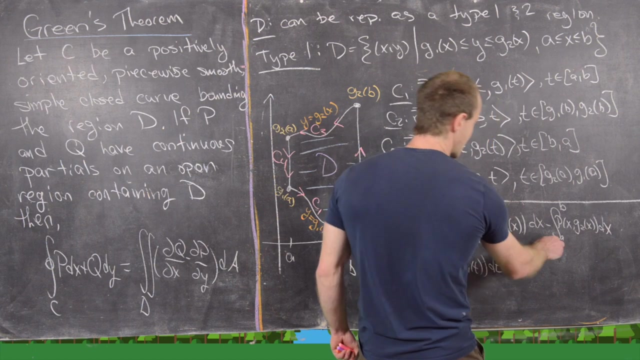 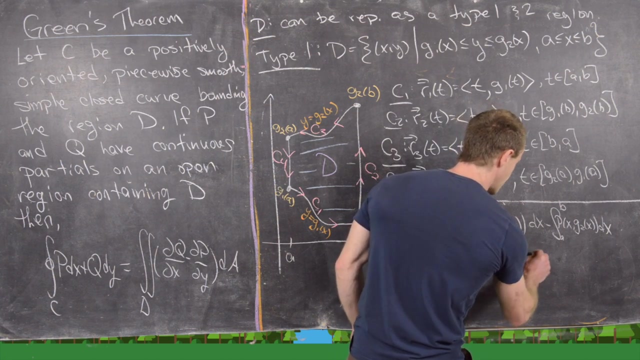 with t's just to really force the fact of what we're doing and notice that this is equal to the integral from a to b of p, of t, g1 of t and then dt. and then i'm going to take that minus sign and switch the order of integration to the integral from b to a, of p, of again t, g2 of t, dt. 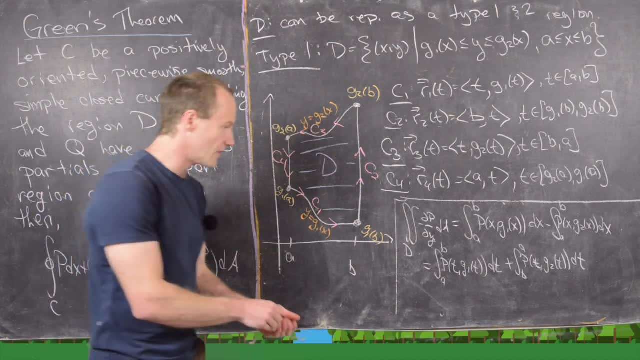 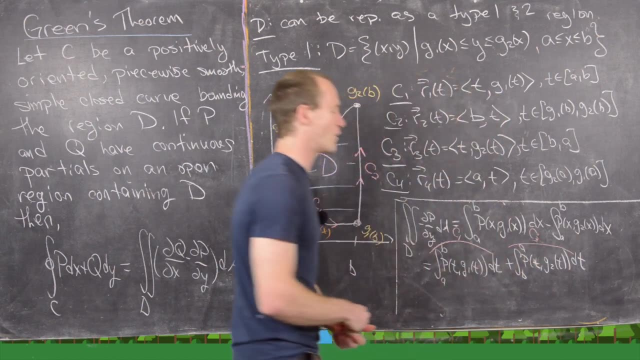 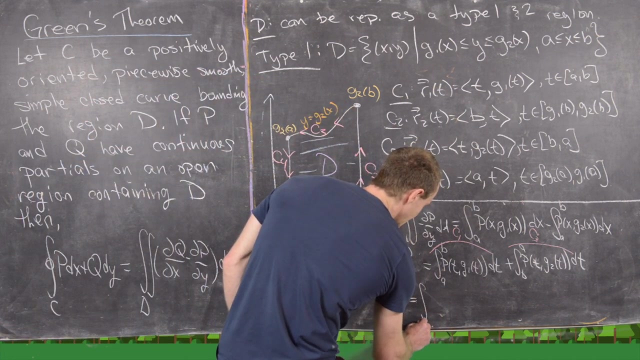 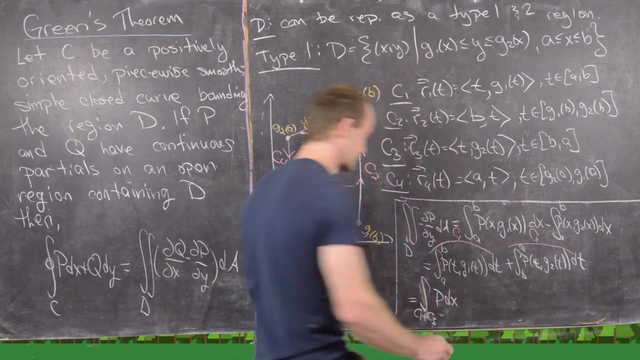 but now notice that this guy right here is just the line integral over c1 and this is the line integral over c3 of p dx. so that means they can add together to be the line integral over c1 plus c3 of p dx. okay, fantastic, now the 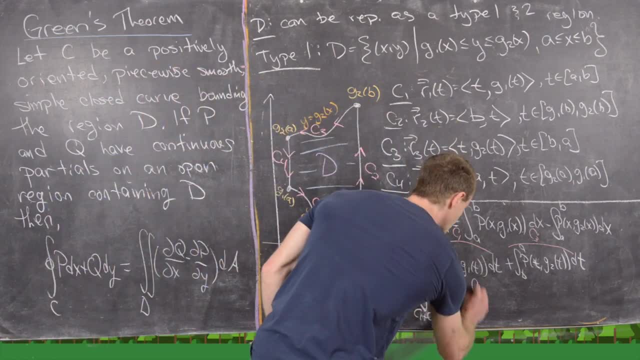 next thing i'm going to do is add zero into this, but the version of zero i'm going to add is going to be the line integral over c2 into the line integral over c3 of p dx, and then i'm going to add zero into this. 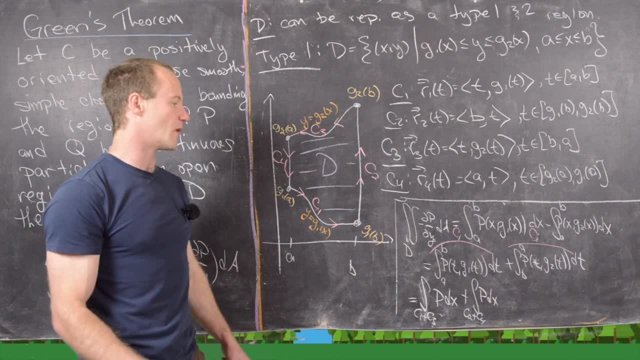 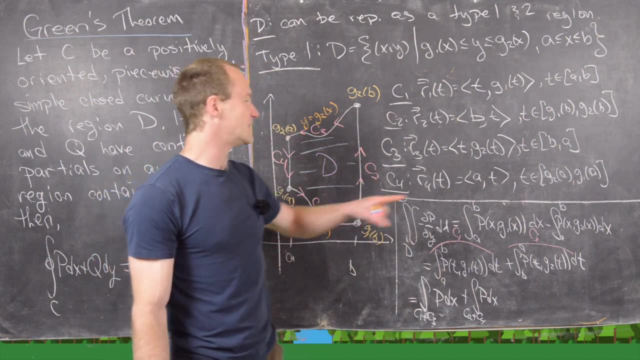 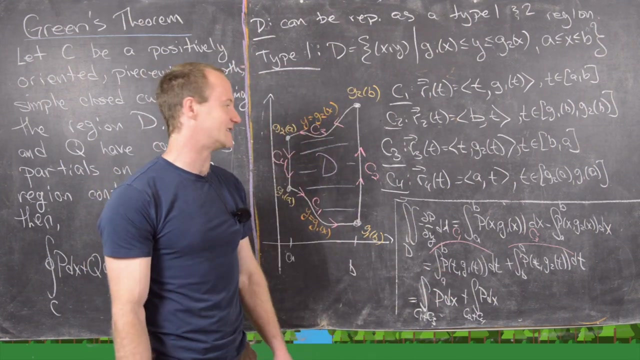 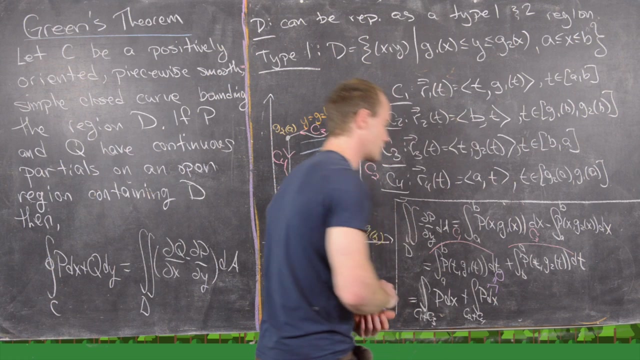 and c4 of p dx. so let's argue why that is zero. so notice: on c2 the x coordinate's never changing. on c4 the x coordinate is also never changing, which means the dx component- which recall that's dx, dt, dt- will always be zero. so let's just point that out here. this thing is always equal to zero. 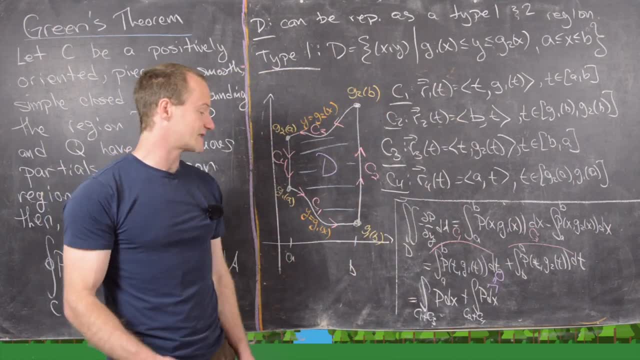 so really we've added zero here. but now notice that we can add zero to the line integral over c2 of p dx, and then we can add zero to the line integral over c2 of p dx and then we can match those two things together to be the integral over c1 plus c2. 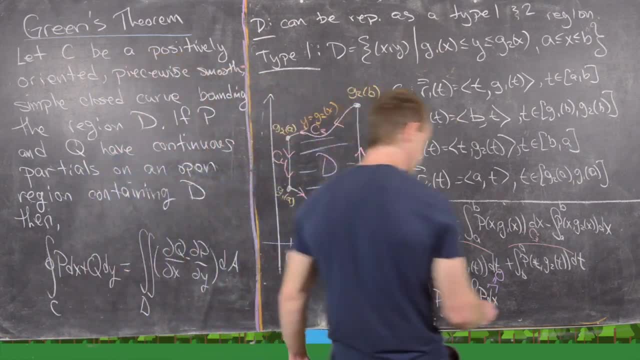 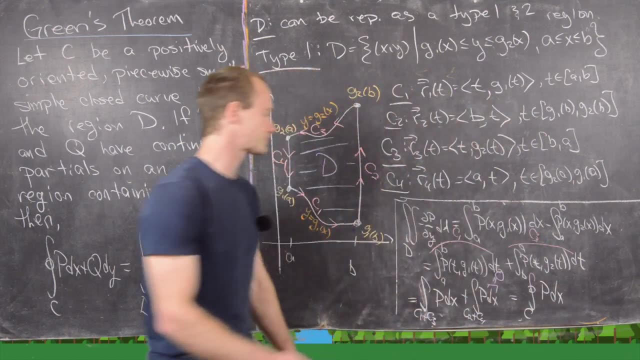 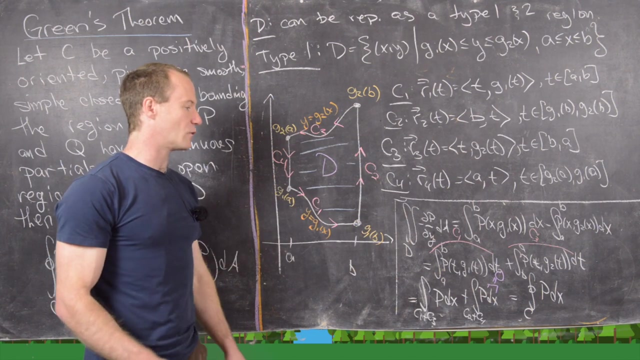 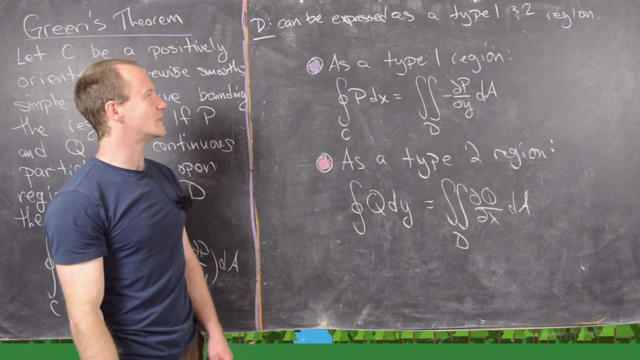 plus c3 plus c4, but that's exactly going to be the line integral over the whole thing c of p dx. okay, great, so now the next thing that i want to do is erase the board, and then we'll summarize what we have and what we can also get from very similar strategies. so what we just did was: